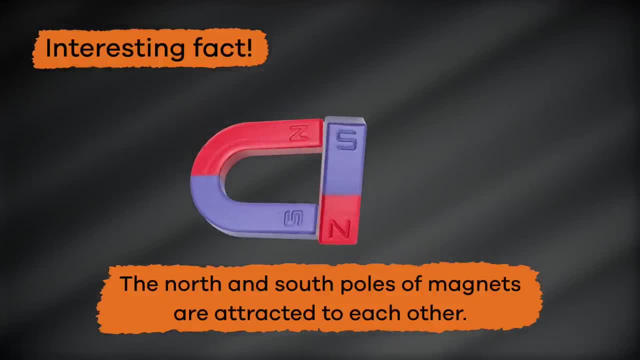 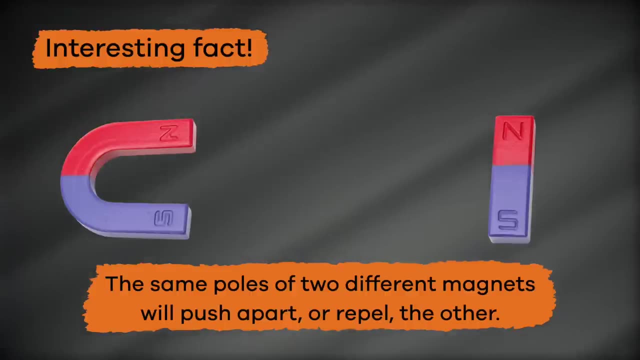 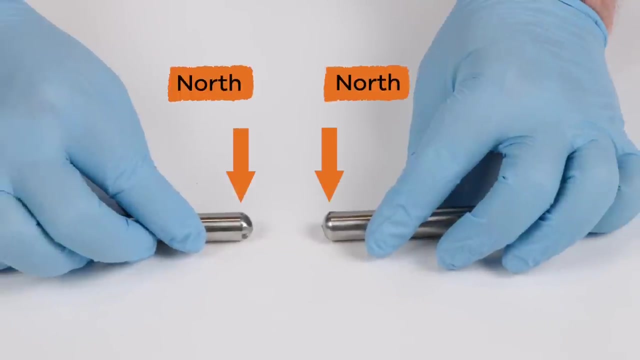 other and will always be pulled towards each other when they are near the other. But the same poles of two different magnets will push apart or repel the other. Let's test this out First. let's try putting two north poles together. Look at that: they are repelling each other. 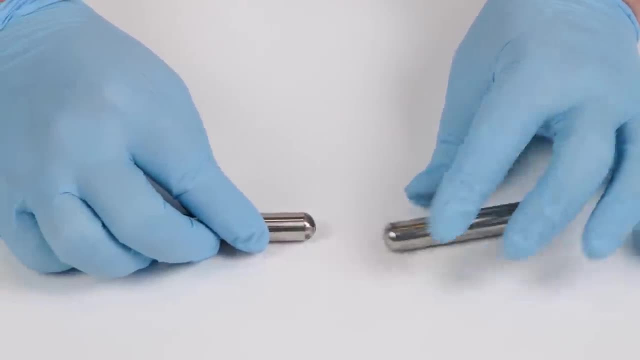 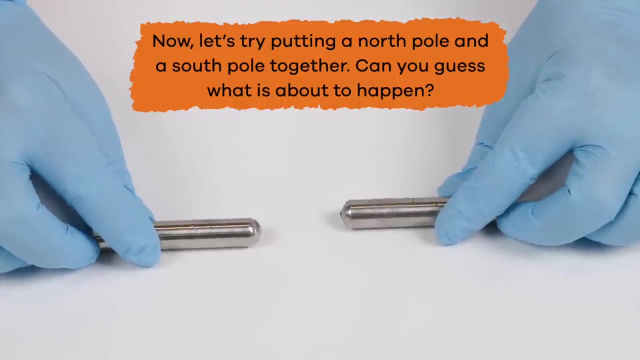 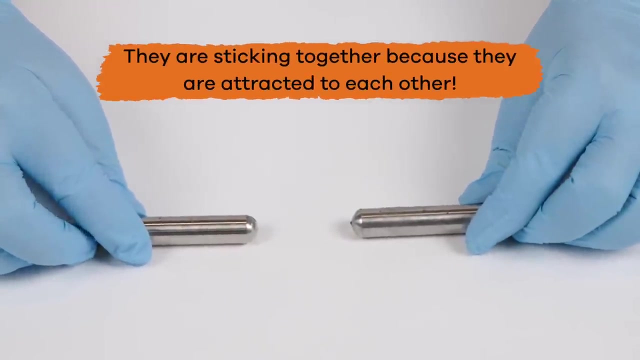 How about two south poles? They also repel each other. Now let's try putting a north pole and a south pole together. Can you guess what is about to happen? You are right. They are sticking together because they are attracted to each other. 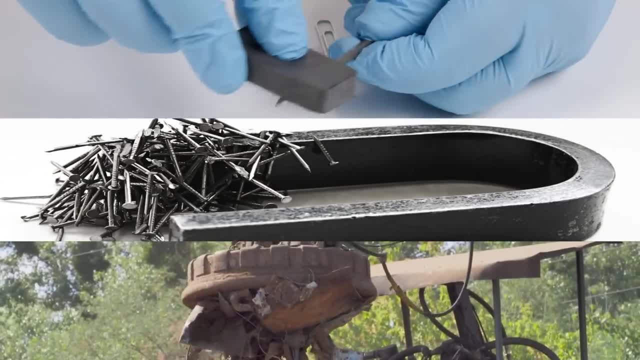 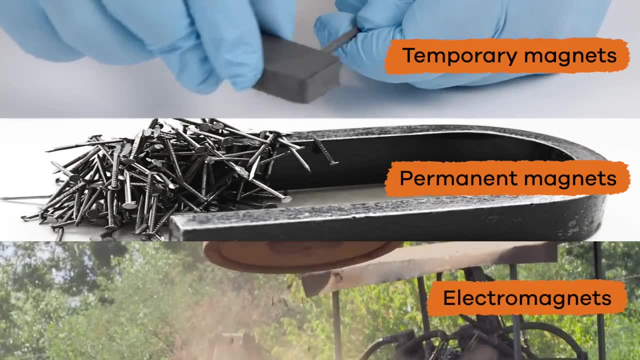 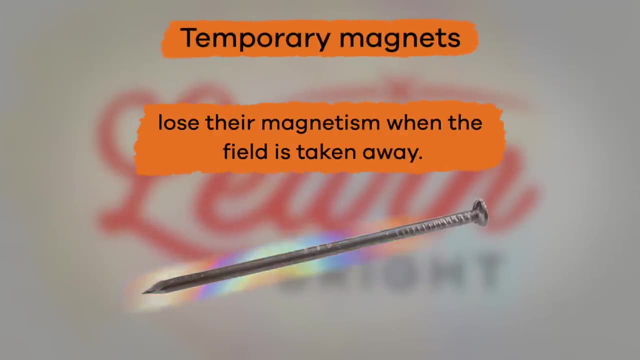 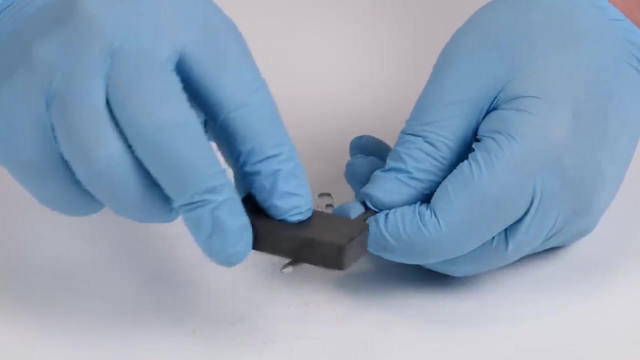 Cool right. There are three different types of magnets: temporary magnets, permanent magnets and electromagnets. Temporary magnets become magnetized when a magnetic field is present and lose their magnetism when the field is taken away, Like when you rub a magnet against another piece of metal like a paper clip or a nail. 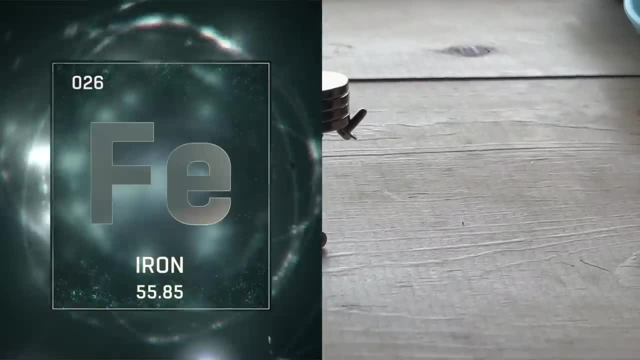 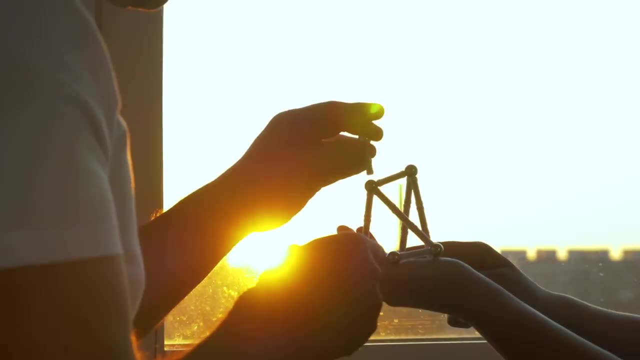 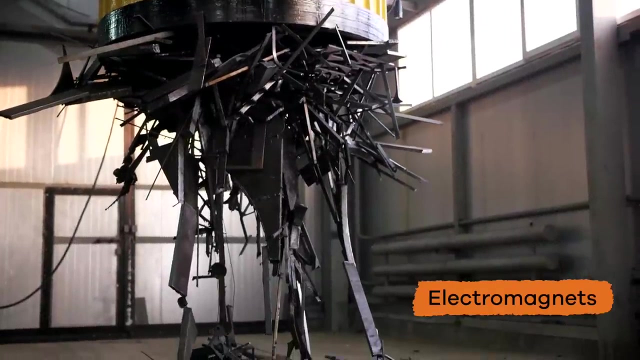 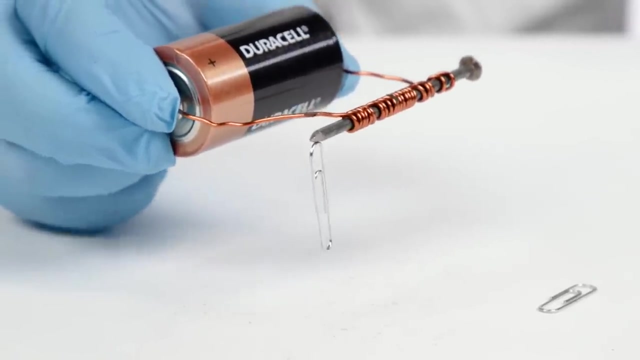 Permanent magnets are made from materials like iron or nickel that are naturally or chemically magnetized and already have their own magnetic fields, like the magnets you use on your refrigerator. Electromagnets are created by magnetization By running an electrical current through a coil with a metal core, the energized core. 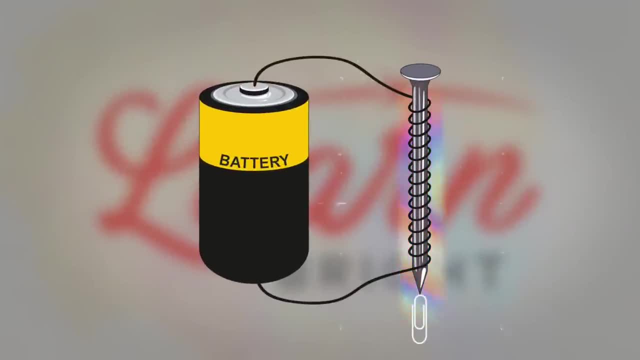 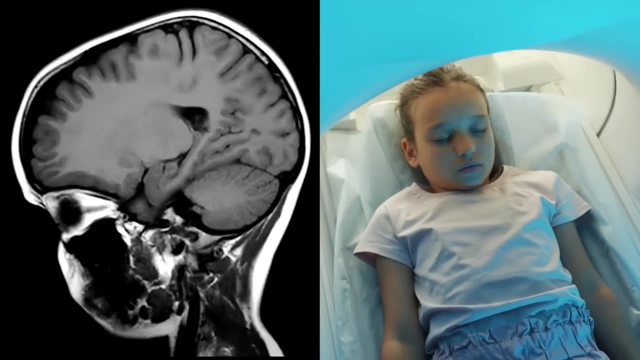 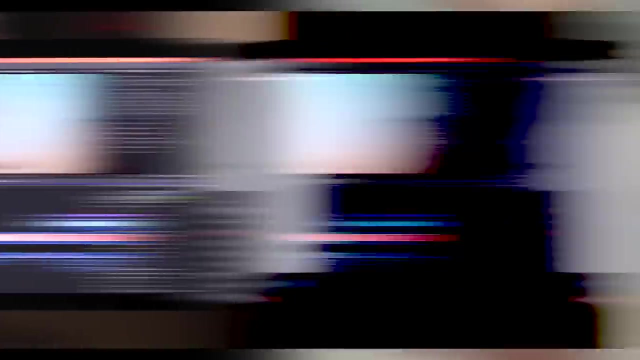 creates a magnetic field, and when the current is shut off, the magnetic field disappears. An MRI machine is an example of an electromagnet. Electronics like TVs and computers also use this kind of technology. Magnets are used in many places for many things. 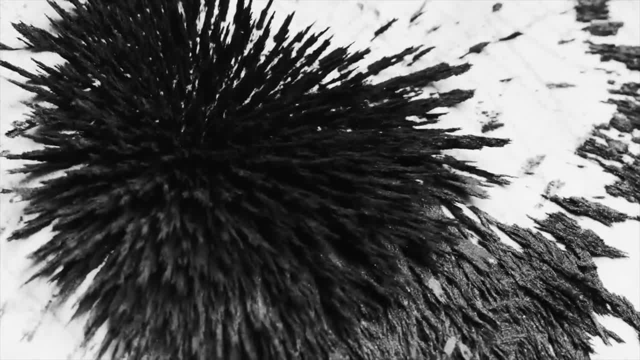 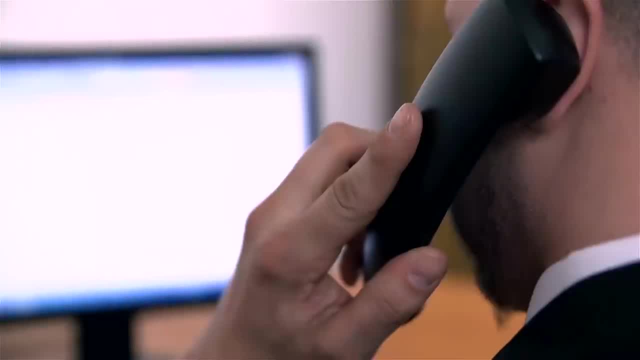 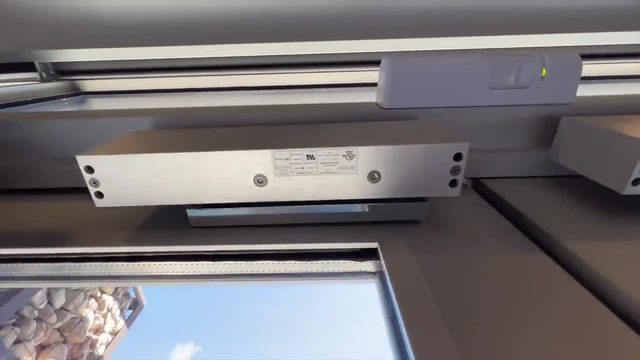 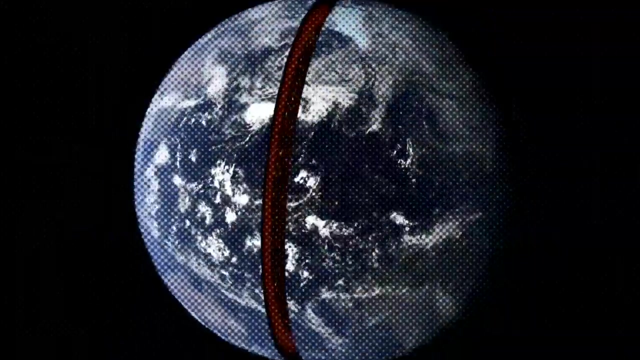 Hang up your schoolwork on the refrigerator. They are used in speakers, computers, motors, doorbells, telephones, compasses and tools. They are also used in doors by recycling centers, hospitals and lots of other places.